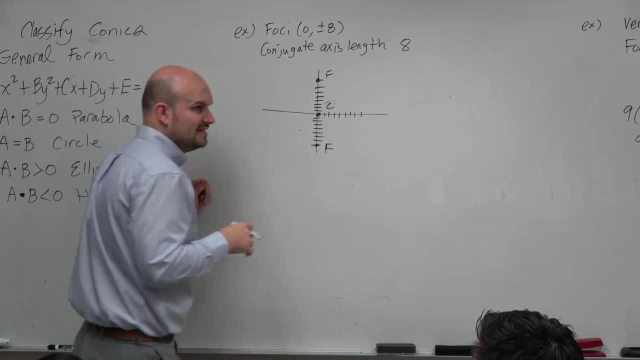 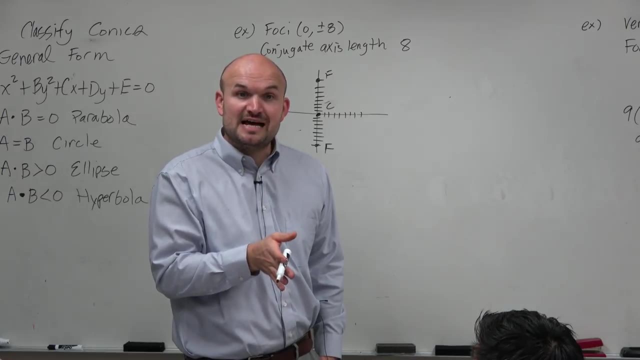 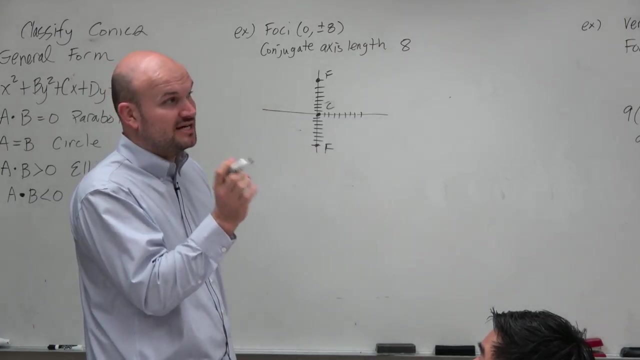 00.. Then also, I know that the foci lie on the. Do we have open seats up here if you guys need We have? the foci lie in the transverse axis. So therefore the transverse axis has to be vertical. And since the transverse axis is vertical, that means my a squared's going. 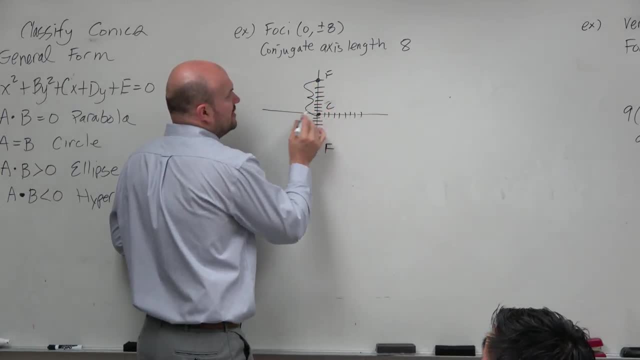 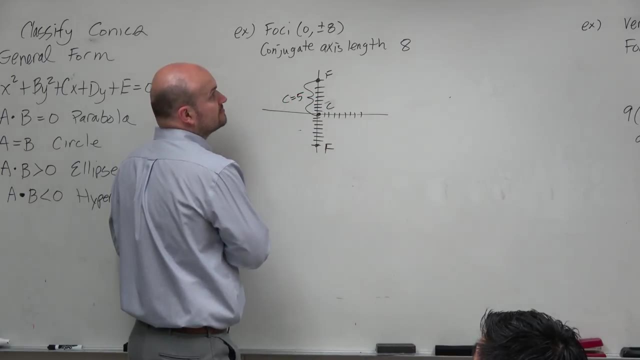 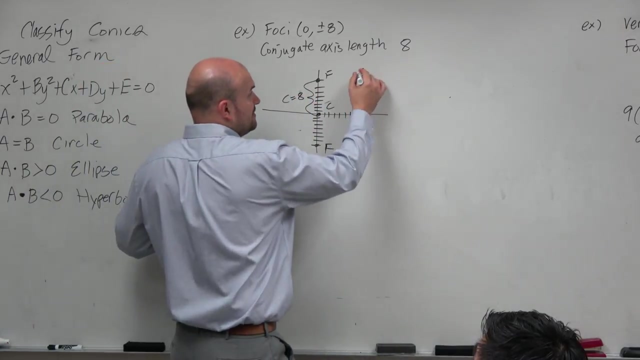 to be under my y. Now again, remember: the distance from center to your foci is going to equal c, which is equal to 5.. I don't know where 5 came from. That's equal to 8.. So if we know c is equal to 8, then we know c squared is equal to 64.. 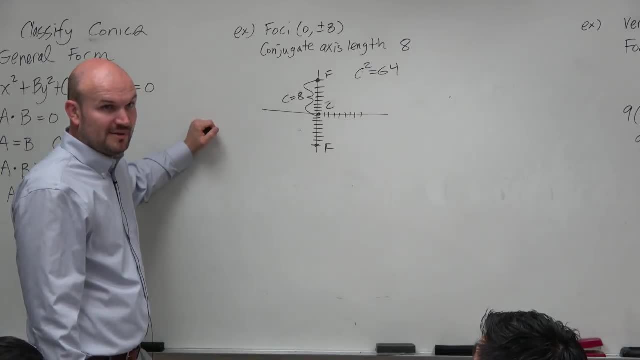 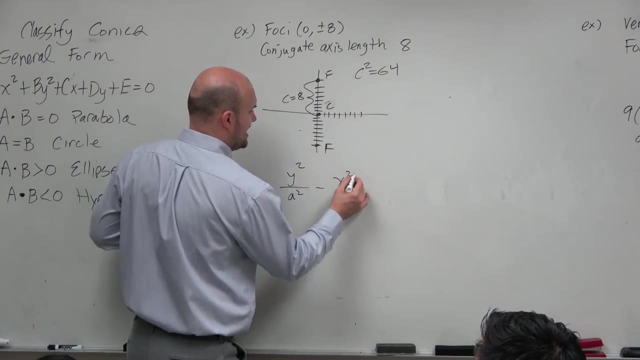 Just from one piece of information, just by plotting this, I'm able to figure out all this information Right. It's quite a bit. So I know that I have y squared over a squared minus x squared over b, squared is equal to 1.. 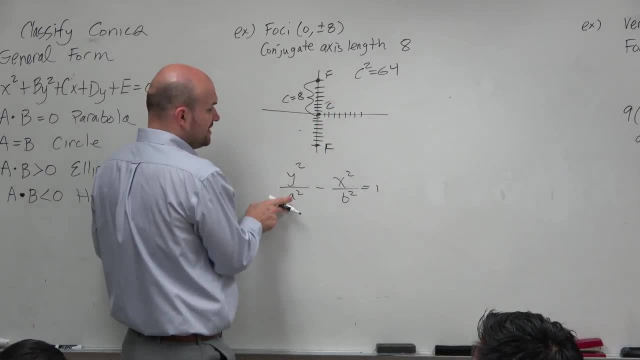 I'm not subtracting h and k because I know h and k are 0.. Now I need to figure out what a squared and b squared is. I only know c squared, So I go to the next one, The conjugate axis length. The conjugate axis is the distance from your co-vertice to your other co-vertice or the distance between your co-vertices And, just like an ellipse, the distance from your center to your one co-vertex is going to be represented by b. 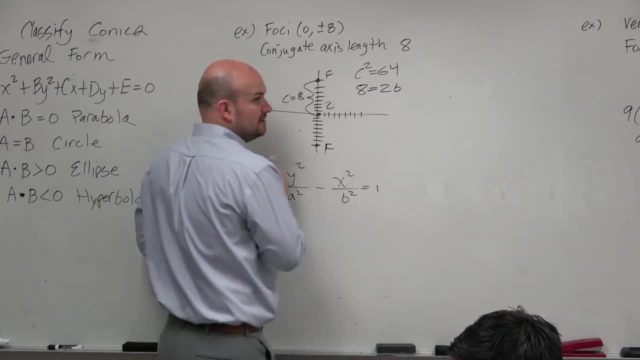 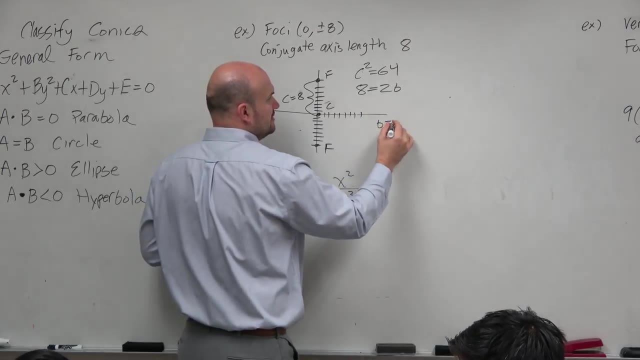 So we can say 8 is equal to 2b. From the center to one. co-vertex is b, So the distance is equal to 2b. The distance from both of them is going to be 2b. So therefore we could say b is equal to 4 and b squared is equal to 16.. 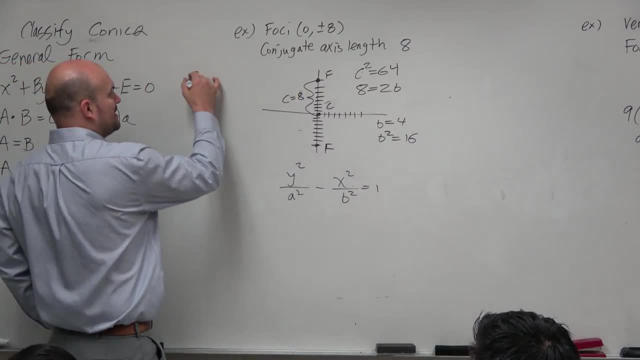 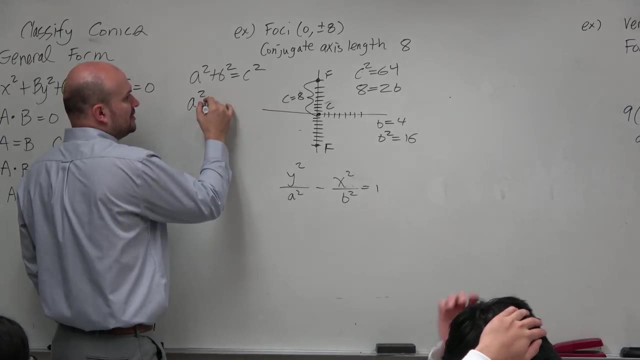 Now to identify what is going to be a, I need to write back my equation. a squared plus b squared equals c squared. I still don't know a squared, but I know that b squared is really kind of getting annoying. And then c squared is going to equal 64.. 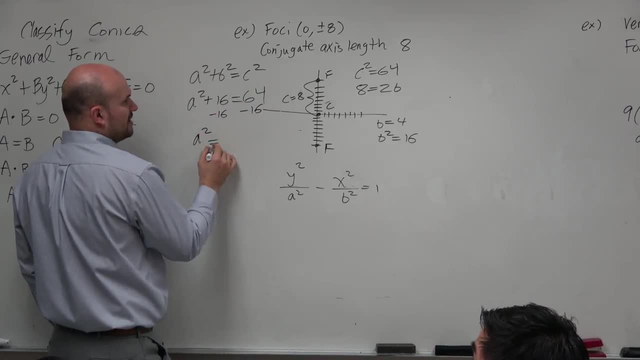 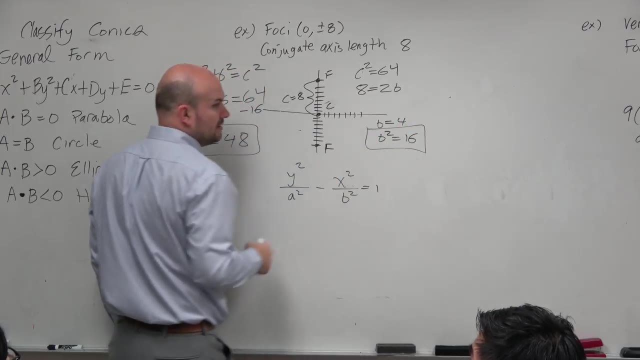 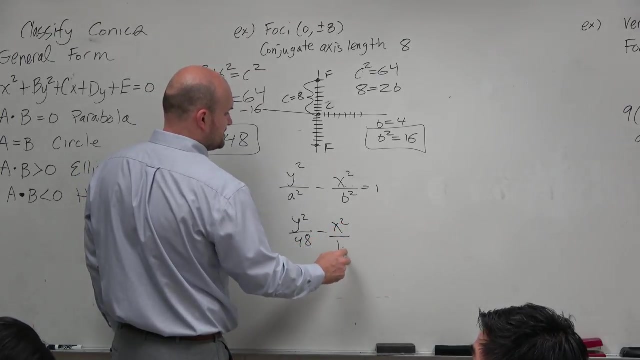 So I subtract, Subtract a squared is going to equal 48.. So now I know a squared And I know b squared, And guys, all I've got to do is now plug it in: y squared over 48 minus x squared over 16 equals 1.. 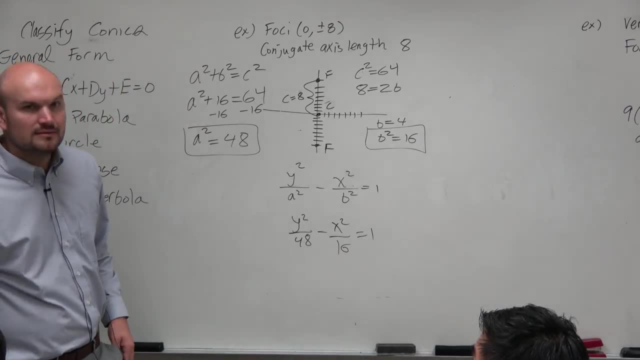 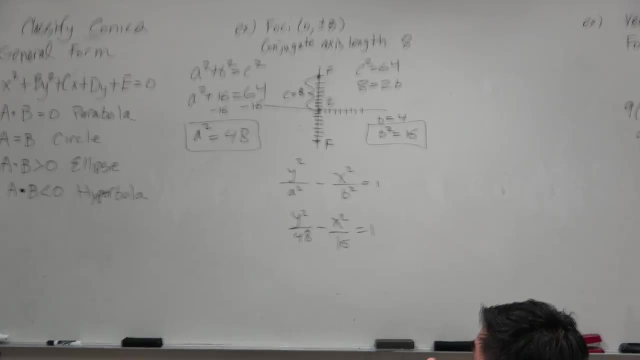 Wasn't that bad, was it? No, It was Painful. Torture Stung just a bit Like a hornet or like a wasp.